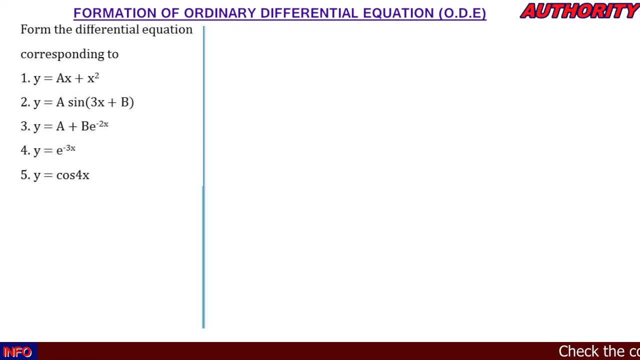 cos 4x. So these are the questions we are going to consider in this video. Alright, please watch carefully and pay attention. It's very simple and it's going to help you. Alright, good, Now let's go. Number 1, we have y is equal to ax plus x squared. You know here. 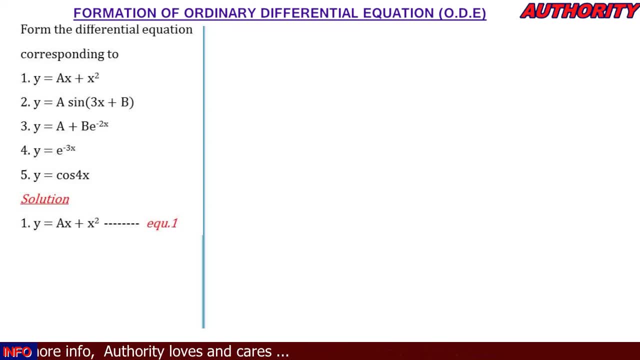 let's take a look at this carefully. We see that we have only one constant. We have a constant. So, as we have one constant, that tells us that we are going to differentiate just once, And then we try our possible best to remove the constant, which is a Alright. 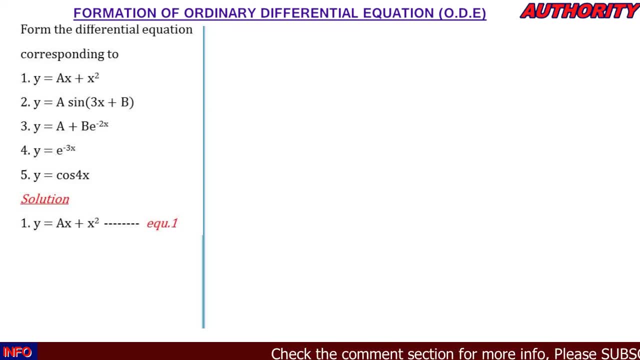 good, Now let's see what we're going to do. We have: y is equal to ax plus x squared. Let's call this equation 1, right? Good, The first thing, let's go. Let's differentiate this for a first time. When we differentiate it for the first time, we're going to have dy dx. 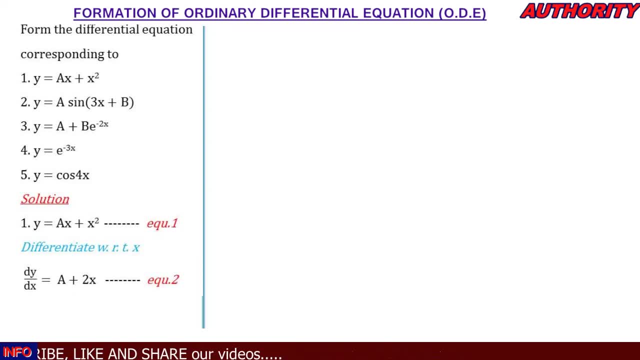 equal to a plus 2x. When we differentiate ax, it's going to give us a, And when we differentiate x squared, it's going to give us 2x. So this is the first derivative. Let's call this equation 2.. Okay, good, Now in this equation 2, we have dy dx equal to a plus 2x. Let's move. 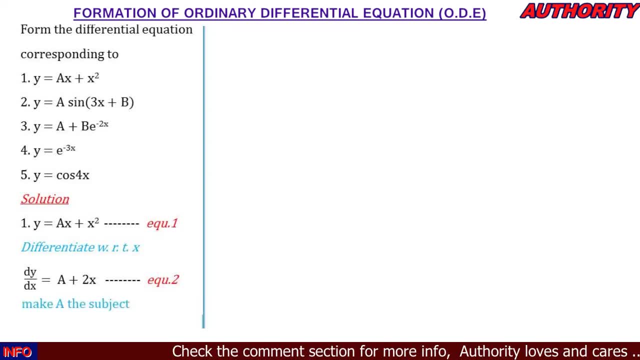 make a the subject. if we try to make a the subject, that means we're going to take 2x to the other side. so when we take 2x to the other side we're going to have dy. dx minus 2x is equal to a. 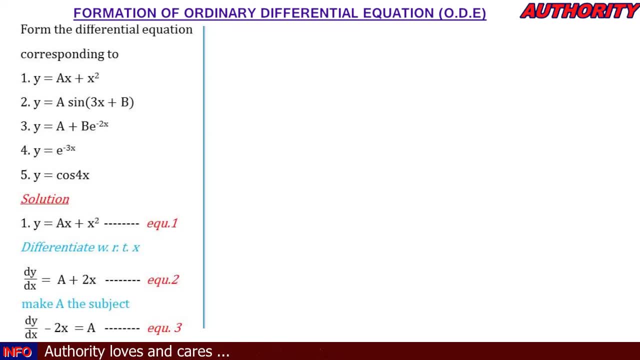 we call this equation three. all right, good now here we know the value for a. okay, we know the value for what for a in this equation three. and then we say that a is equal to dy dx minus 2x. let's substitute this into equation one. you know, in equation one we have 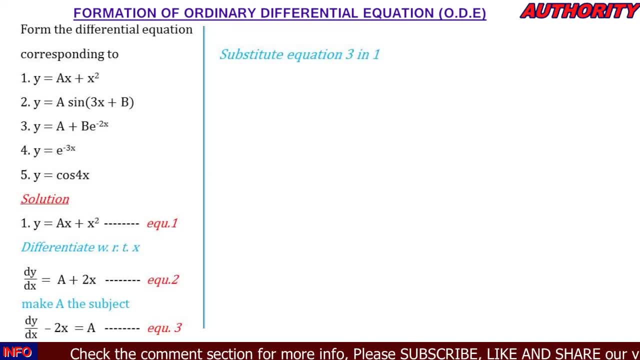 y is equal to ax plus x squared. and now we know the value for a, so we can replace the value for a in equation one. now let's do it again. so let's go. equation one we have: y is equal to ax plus x squared, so in place of a, let's replace it. 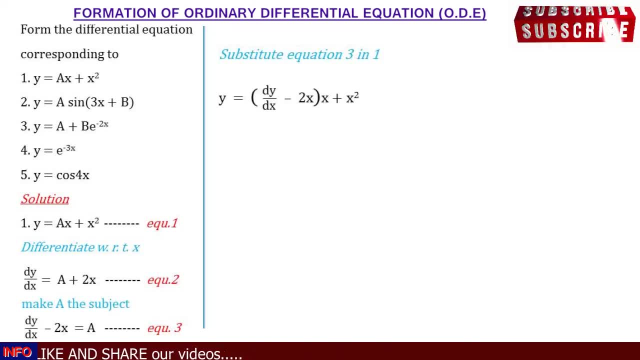 with this value that we have now. okay, so that means we're going to have: y is equal to dy dx minus 2x in bracket x, plus x squared. okay. so let's use this x to open the bracket. we'll have x multiplied by dy dx. we're going to give us dy dx in bracket x and then we will say x. 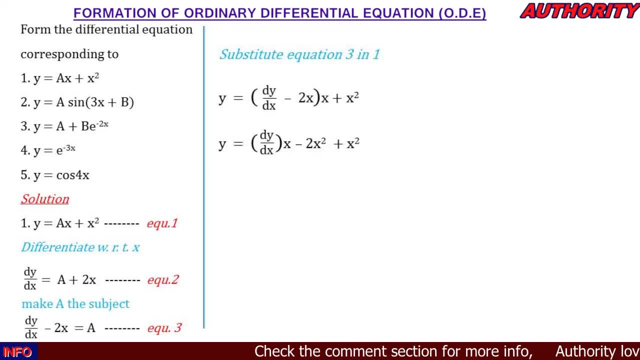 multiplied by dy dx minus 2x, plus x squared. okay, so let's use this x to open the bracket by minus 2x is going to give us minus 2x squared. then we have plus x squared, all right. good, we have minus 2x squared plus x squared. so when we say minus 2x squared, plus x squared is going to give 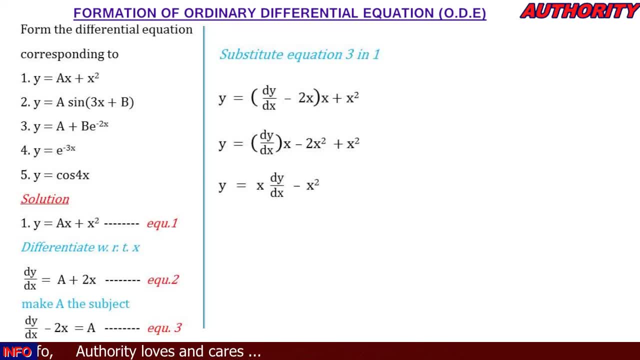 us minus x squared. so here we have: y is equal to x, dy dx minus x squared. from here, let's move everything to one side and rearrange them based on the number of degree. okay, so when we move and rearrange, we're going to have x, dy dx minus x squared, minus y equal to zero. 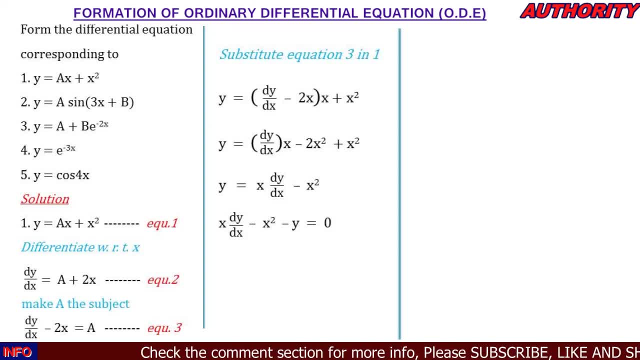 here we have. what x, dy, dx minus x, squared minus y, equal to zero, right? good, please? i want you to solve this by yourself, you, and see if it will give you the same result. now let's see number two. number two here we have: y is equal to a sine 3x plus b. all right, here we have two constants. 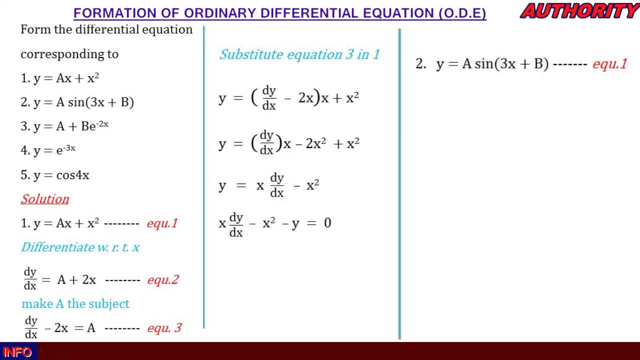 involved. that means we're going to differentiate these two times. okay, now let's call this equation one. so we have: y is equal to a sine open bracket, 3x plus b. let's differentiate this for the first time. we will differentiate it. for the first time, we're going to have dy dx equal to in the right hand. 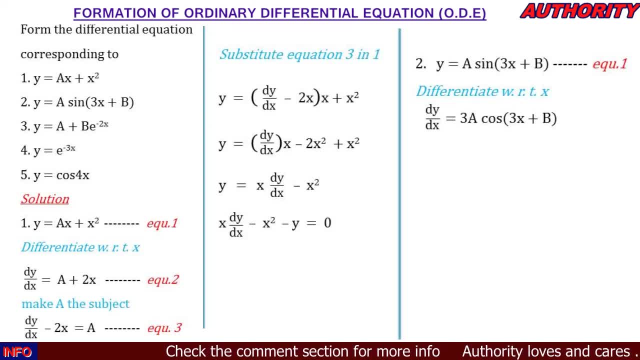 side, we're going to have 3a cos, 3x plus b. hello, i know some of us may be confused here, but if you know your differentiation very well, you see that you'll not be confused yet. okay, so we have lessons on differentiation, we have our product rule, chain rule, quotient rule and all that. please don't forget to subscribe to our channel and hit the bell icon so you don't miss any of our new videos, and we'll see you in the next one. bye, bye, bye. 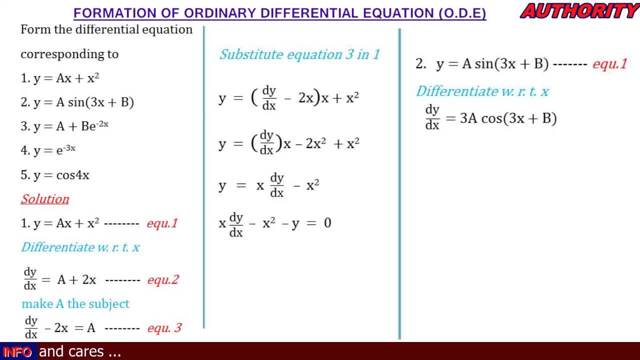 i want you to study them very well before diving into ordinary differential equation. it should be very simple. if you revise your differentiation, okay, good, please. this is what you have. you differentiate sine 3x plus b using chain rule. that is, you're going to say let. 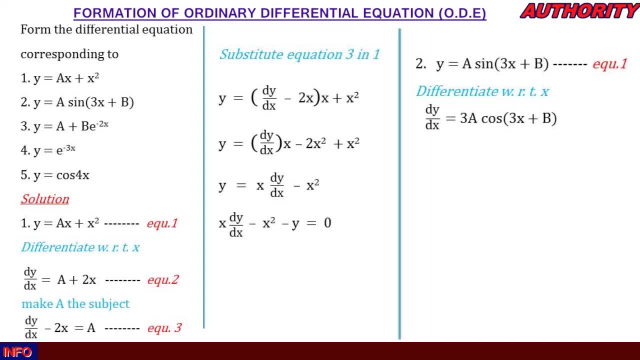 everything in the bracket 3x plus b. let it be called a letter, maybe t, and then you differentiate that one different and then differentiate the new sine t different. you get it. you know the way you do it. now let's go. we have dy. dx is equal to 3a cos 3x plus b. 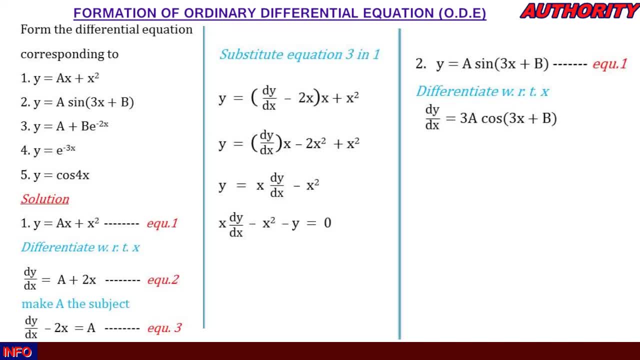 is that true? yes, now we call this equation true. let's differentiate this again. we'll differentiate this for the second time. we're going to have d squared y all over d, x squared equal to. we're going to have d squared y all over d, x squared equal to. 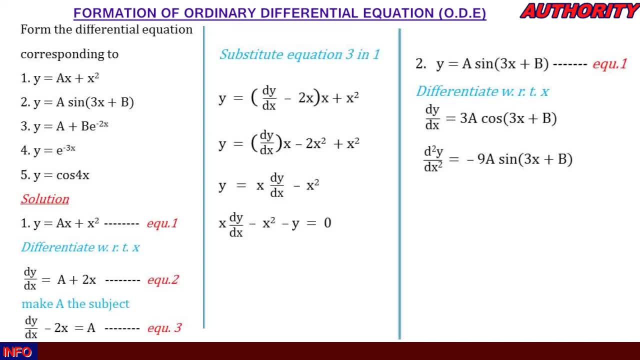 minus 9a sine open bracket, 3x plus b. the same thing we did in the first. differentiation is the same thing we did here. but in this time around we have cos x and when we differentiate cos it's going to give us negative. so we have minus 9a sine open bracket, 3x plus b, all right. 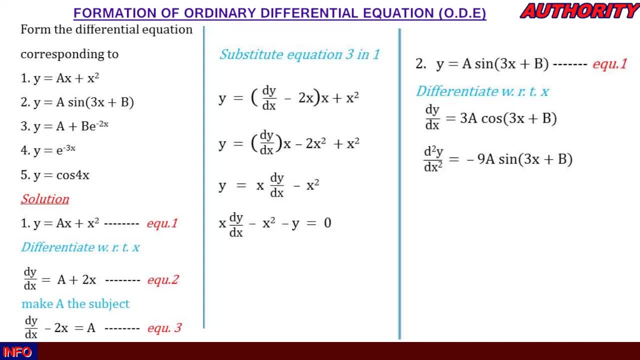 yes, now in this equation, in this last equation, let's call it equation three. so in this equation three, if you look at it very well, it looks similar to equation one. so, but the difference is minus nine. let's factor out minus nine and put it in one side. 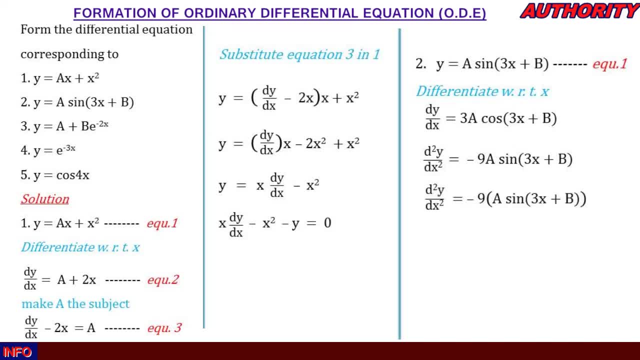 we're going to have d squared y all over, b x squared is equal to minus nine in bracket a sine 3x plus b, minus nine. open bracket a sine 3x plus b. all right, yes. so here we have a sine 3x plus b, which is the same value that we have in equation one. so we're going. 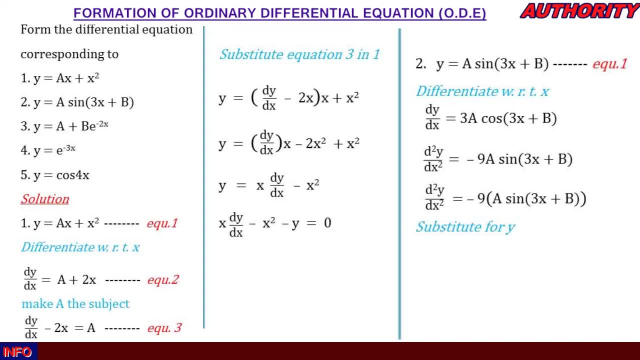 to substitute for y. so in place of a sine 3x plus b, we're going to replace it with y. so we're going to have d squared y all over d, x squared equal to minus nine, y, because y is equal to a sine 3x plus b. so let's take minus nine and put it in one side, so we're. 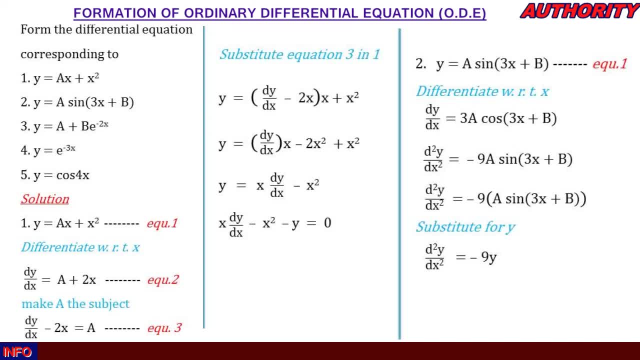 going to substitute for y. so in place of a sine 3x plus b, we're going to replace it with a sine 3x plus b. so let's take minus nine y to the other side. we're going to have d squared y all over. d x squared plus nine y is equal to zero. all right, yes, this is the. 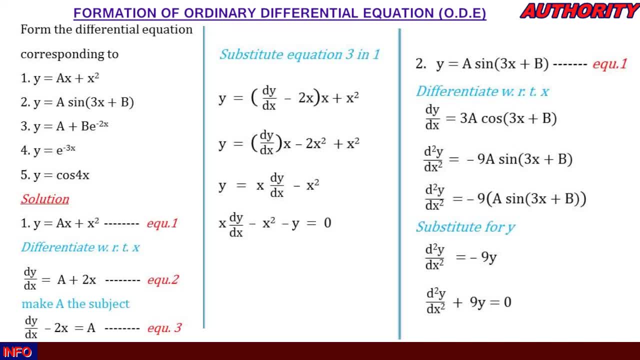 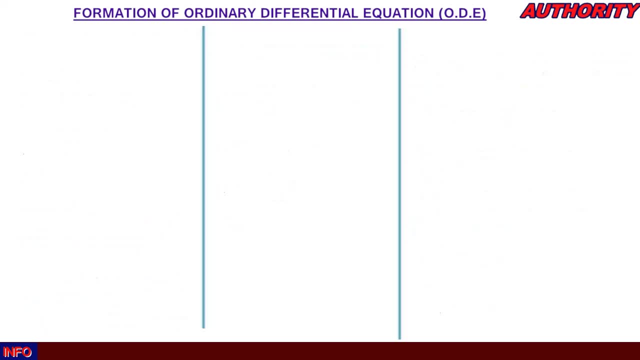 differential equation corresponding to y is equal to a sine 3x plus b. all right, yes, let's go number three. number three we have: y is equal to a plus b, exponential minus two x's. let's pay attention to this. how many constant do we have? we have two, a and b, right, good? 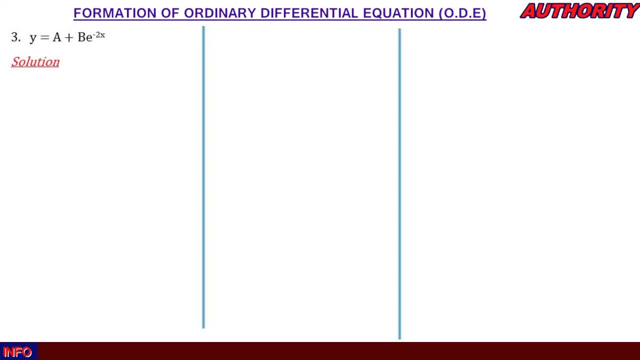 let's try to eliminate this. a and b, that means we're going to differentiate two times. so the first time, let's call this equation equation one. y is equal to a plus b, exponential minus two x. let's call it equation one. let's differentiate for the first time. when we differentiate, we're. 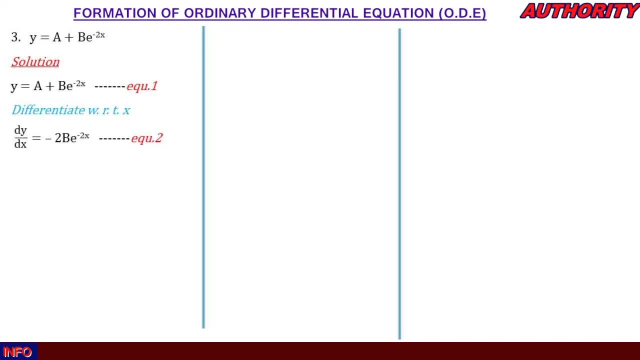 going to have d, y, d, x is equal to: when we differentiate a, it's going to give us zero. and then we'll differentiate b exponential minus 2x, it's going to give us minus 2, b exponential minus 2x. is that true? yes, good, so we call this equation two. so the first differentiation. 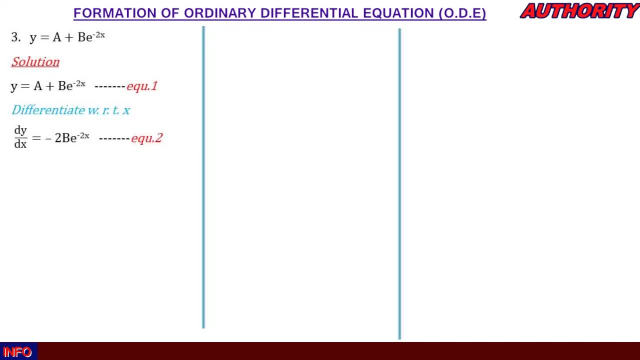 or the first derivative we have: d, y, d, x is equal to minus two b exponential, minus 2x. okay, good, let's differentiate this again. that is the second time we're going to have d squared y all over d, x squared equal to when we differentiate minus 2 b exponential. 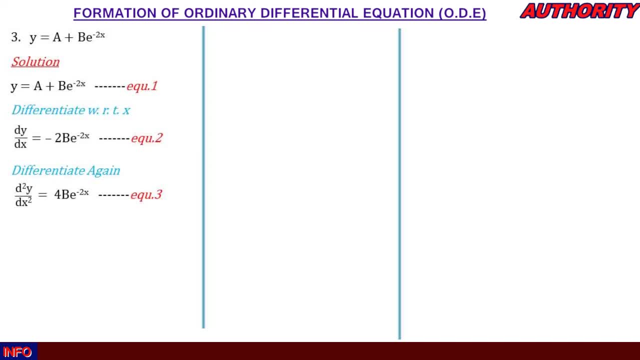 minus 2x. you know, this minus 2 is going to come down and multiply minus 2. okay, now, when you have minus 2 times minus 2, it's going to give us plus 4, and then we have b exponential minus 2, x. is that true? yes, so we call this equation three. so equation three. after when? 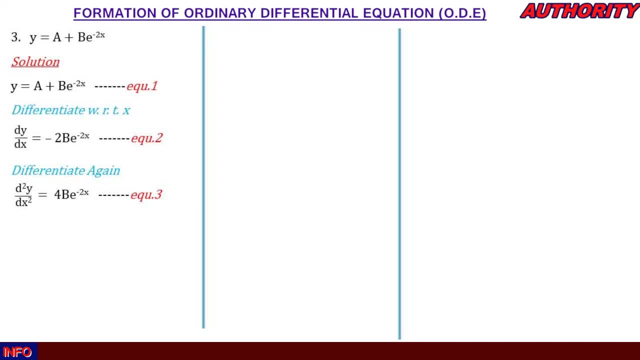 we differentiate the second time, we have d squared y all over d, x squared equal to 4 b exponential minus 2 x. this is how i write. good, let's see what we're going to do again in this equation three. let's write this equation three like this: 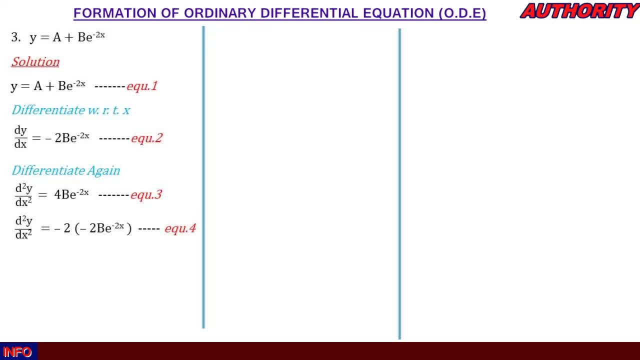 the square y all over d square equal to minus 2 Open brackets minus 2 B exponential minus 2. you know, when you say minus 2 times minus 2 B exponential minus 2x is going to give you the same thing in Equation three. is that true? yes, 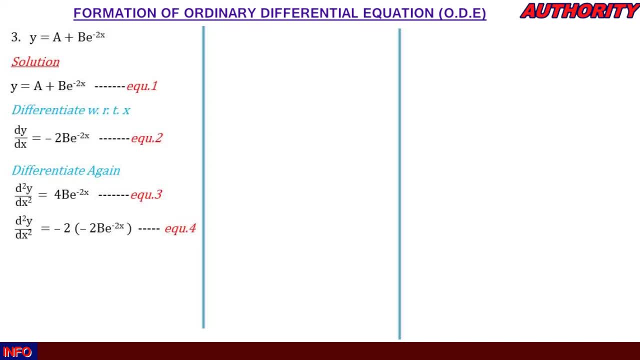 now, as spend this into two, we discovered now we are having a, exactly the same value that we have in equation two: G, eleo IQ. we have in equation what: 2.. In equation 2 we have dy: dx is equal to minus 2 b exponential. 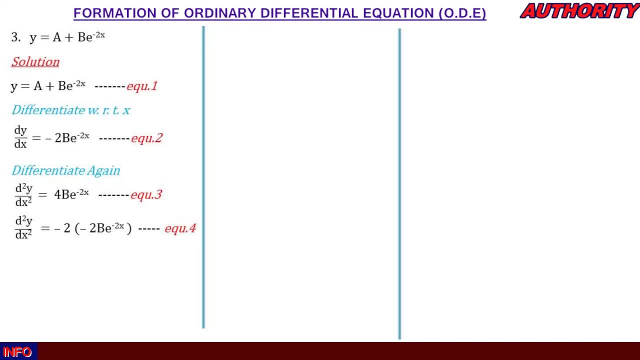 minus 2 x. and then in equation 4, here we have d squared y all over, dx squared equal to minus 2 open bracket: minus 2 b, exponential minus 2 x. So in the place of this minus 2 b, exponential minus 2 x, we can replace it with the value we have in equation 2.. That means here we're going. 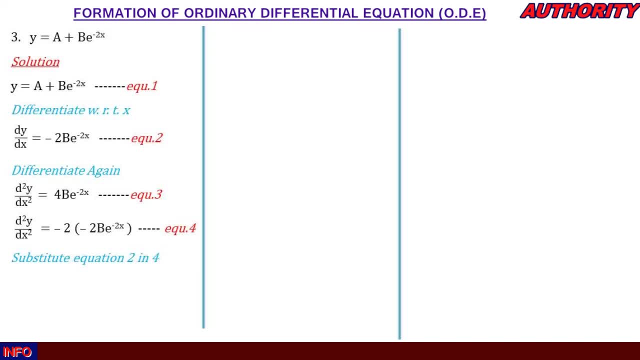 to substitute equation 2 in equation 4.. Okay, we're going to replace minus 2 b exponential minus 2 x with the value we have in equation 2.. So when we do so, we're going to have d squared y all over dx squared equal to minus 2.. 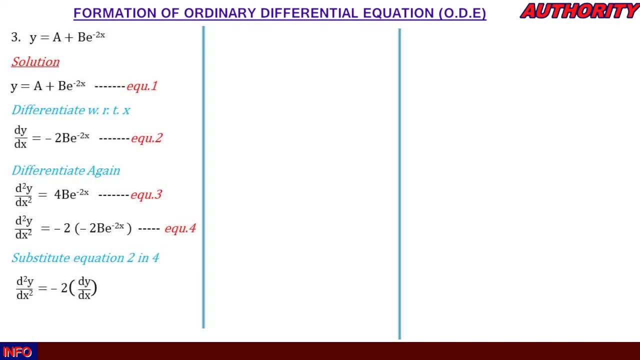 Open bracket. in place of minus 2 b, exponential minus 2 x, we replace it with dy dx. Okay, good, Now, as we replace it, let's remove the bracket. That means we're going to have d squared y all over dx squared equal to minus 2 dy dx. Let's take this to the other side. We're going. 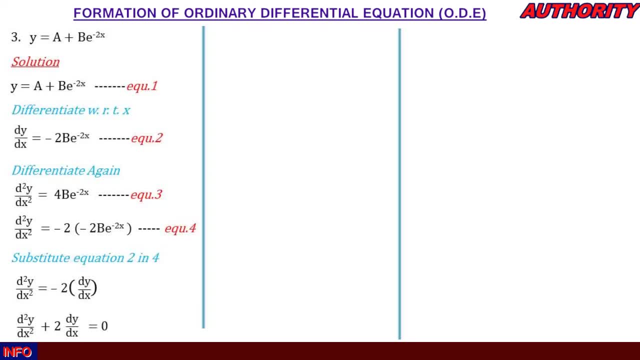 to have d squared y all over dx squared plus 2.. So this is the differential equation of the function. y is equal to a plus b, exponential minus 2 x. All right, Yes, Let's take number 4.. Number 4 we have, y is equal to exponential. 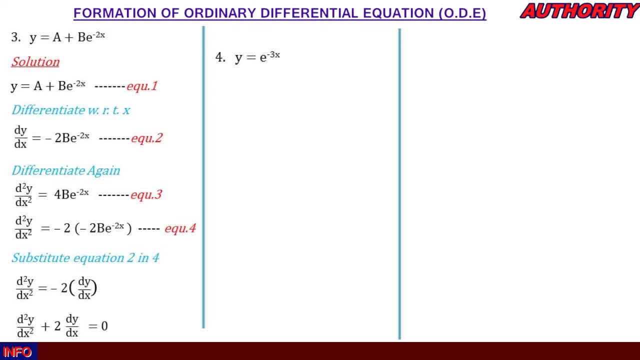 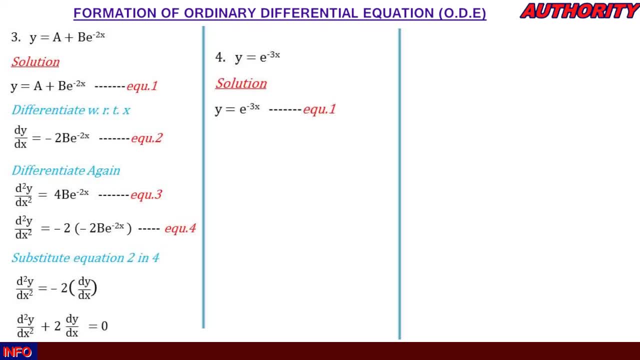 So let's call this equation 1.. Let's call this equation 1.. Now let's differentiate. When we differentiate, we're going to have dy dx equal to minus 3 exponential minus 3 x. Minus 3 exponential minus 3 x. 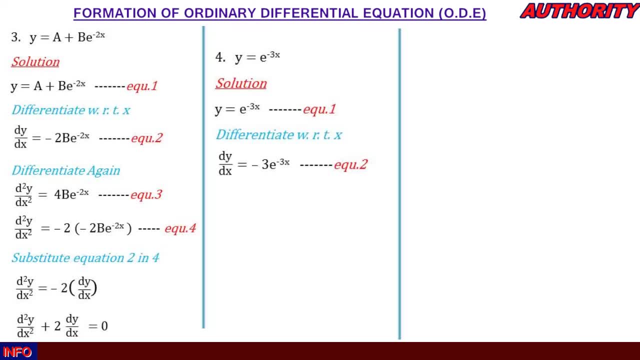 Okay, good here, let's call this equation 2. okay, as we call this equation 2, let's factor minus 3 out. now here we're going to have dy: dx is equal to minus 3, open bracket exponential minus 3x. we'll call this equation 3. so we'll look at this equation 3 and equation 1. they are almost the. 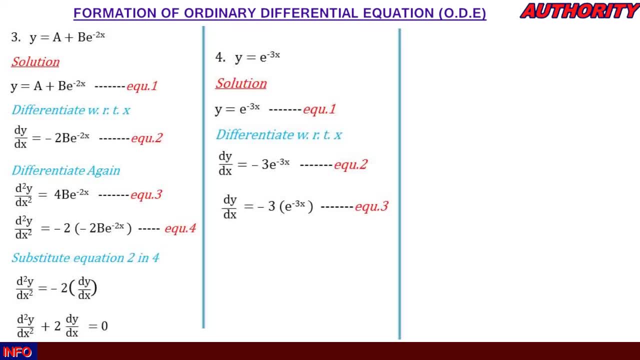 same. so here we're going to replace exponential minus 3 with another value found in equation 1. that means we're going to substitute equation 1 into 3. okay, so here we're going to have dy. dx is equal to minus 3y. so we replace exponential minus 3x with y, because in 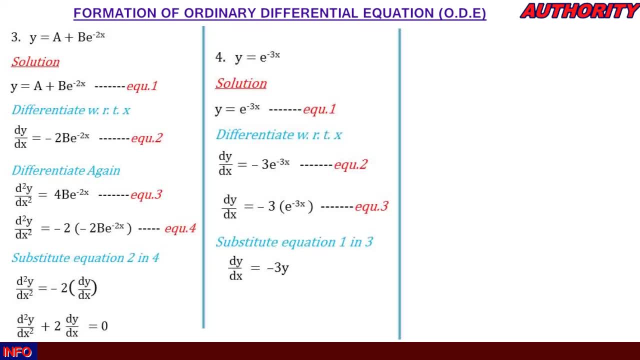 equation 1, we say that y is equal to exponential minus 3x. okay, so as we replace it, we have dy dx is equal to minus 3y. let's take minus 3y to the other side. we're going to have dy dx plus 3y is equal to 0. all right, yes, now let's take the last one number. 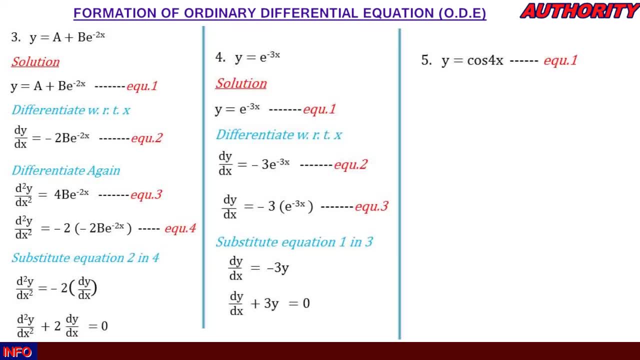 5 we have: y is equal to cos 4x, y is equal to cos 4x. so let's call this equation 1. okay, good, let's differentiate this for the first time. when we differentiate this for the first time, we're going to have dy: dx is equal to minus 4 sin 4x. hello, we're going to have minus 4 sin 4x. 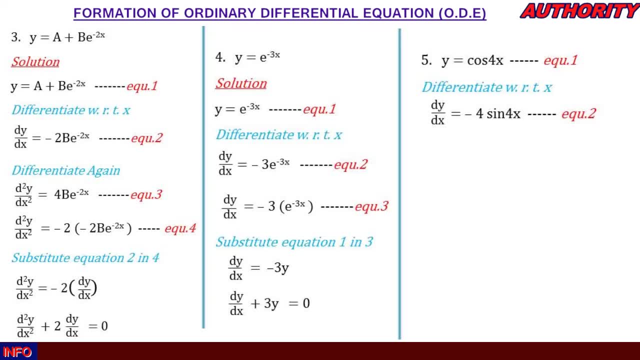 now, if we want to differentiate this cos 4x, we're going to replace 4x. we're going to say let 4x be called the letter t. that means we're going to have cos t now in that place. you say: let t equal to 4x. differentiate t with respect to x. that's going. 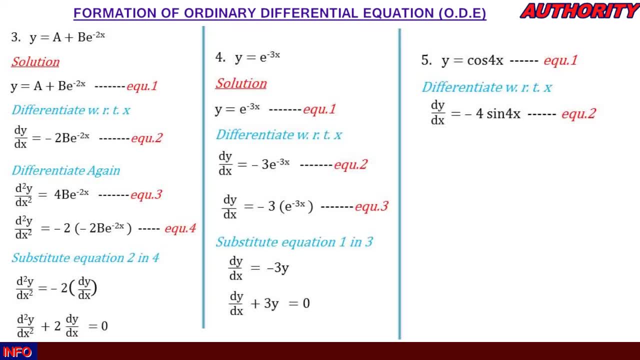 to have 4 and then, when you differentiate cos t, you're going to give us minus sin t. you get it. so that is, you differentiate the function y with respect to t, you get it. and you differentiate t with respect to x when you bring the two differentiation together or the two derivative. 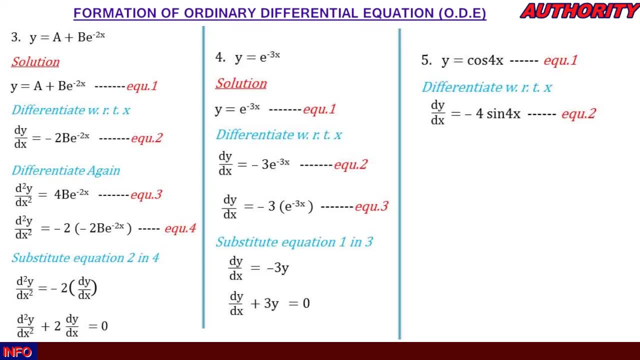 you are going to have d y over the x is equal to d y over the t times the t over the x. so you multiple both of them together is going to give you minus 4 sin 4x. is that clear? now let's continue here. we have d y over the x is equal to minus 4 sin 4x. let's differentiate.